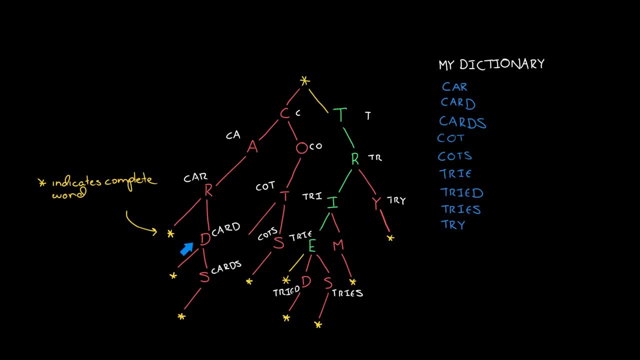 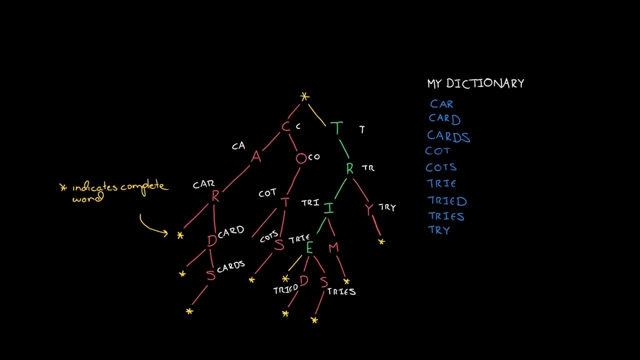 also card, So car is also a prefix, So it allows us to do very fast lookups. So let's talk briefly about the implementation of it. So we're going to need a class node and then, rather than having, as we would in a binary search tree, a pointer to the left and 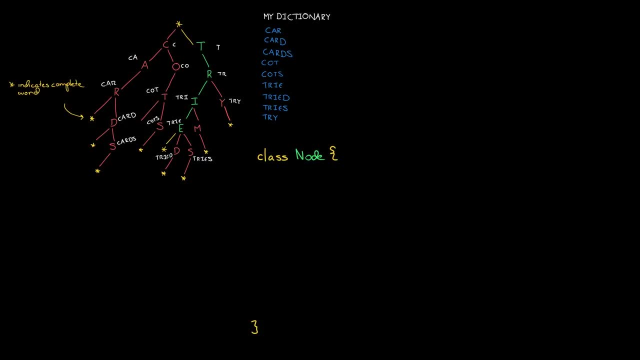 right node. instead, we have some sort of either array of all the children or, more likely, some sort of lookup table that maps from a character to that node. So we can immediately say: do you have a child that is an A Great? give me that immediately. Additionally, we need to. 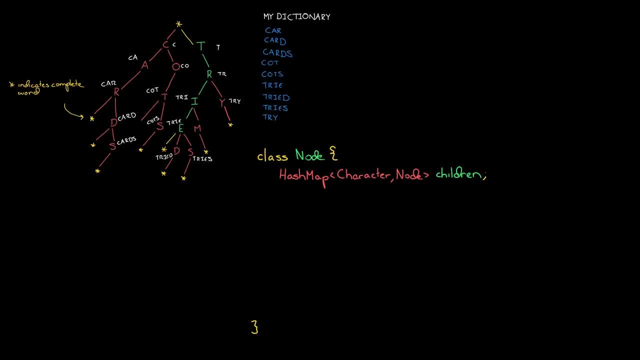 understand. not just is there a, do you have an R as a child, an R node as a child, but is that actually a complete word or is it just a prefix? And so, in addition to each node having a mapping of character from character to node, each node also has some sort of flag in it, called something. 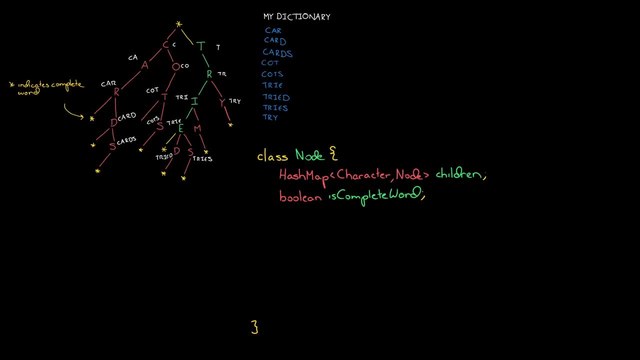 like isComp complete word that represents. is that a complete word or not? We see tries in a lot of problems. So if you're in an interview and you get a question that has some sort of word validation to it, so check if this is, walk through this table and find all the 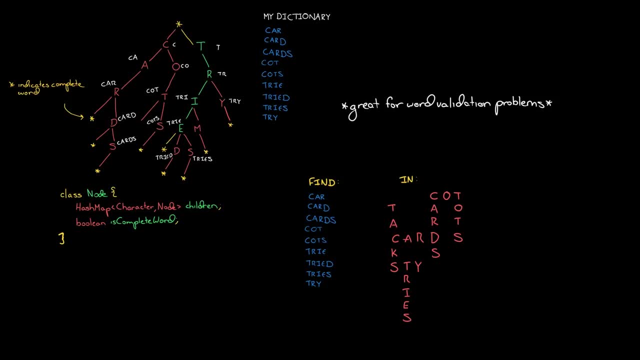 walk through this Scrabble board and find all the words or, given this list of strings, find all celebrity names. So when you see something that has some sort of word list validation, think about whether or not a try might be useful. There's one optimization that often comes up in try problems. Suppose you had a situation where 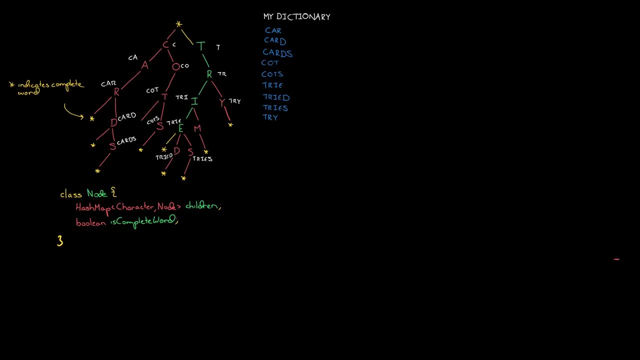 a user was typing a word and as soon as the word became- and clearly was going to be an invalid word, you want to say: underline it. So someone types C and you say, yes, that is in fact potentially going to be a valid word. And then someone types CA. okay, great, we're looking good. 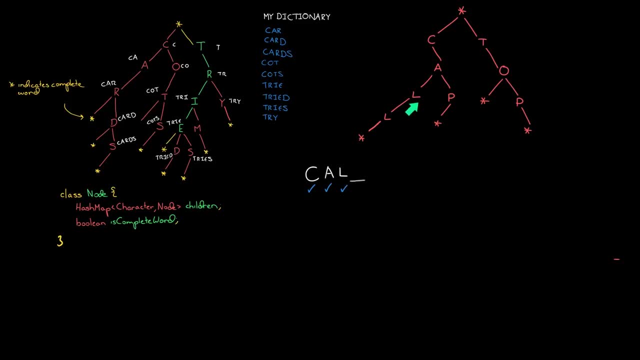 The type CAL. yes, okay, there's words that start with CAL, Now the type CALP. oops, no, that's an error. So that's a good place to use a. try Now the way that I've explained. try so far.